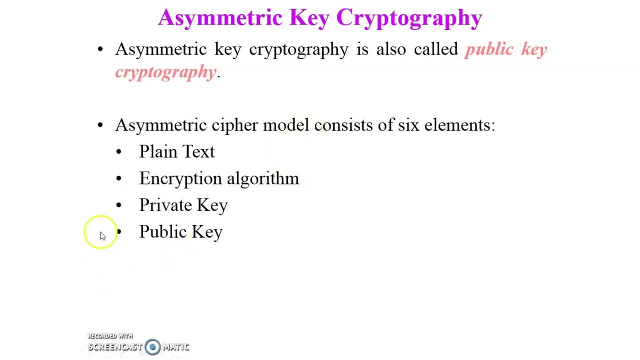 encryption algorithm: private key and public key. This is the key pairs. Fifth, one is cipher text and next is decryption algorithm. So these are the essential ingredients of the asymmetric cipher model and all the definitions of these elements are already discussed in basic terminology of the network security video. 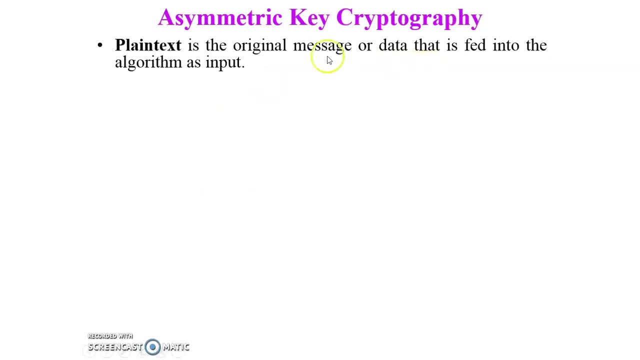 First one, plain text, is the original message or data that is fed into the algorithm as input. So original message, which is sender wants to send to receiver. that message is known as plain text. Second one is Encryption algorithm. So it performs various transformation on the plain text. So encryption algorithm is one kind of technique in which input is plain text and key. 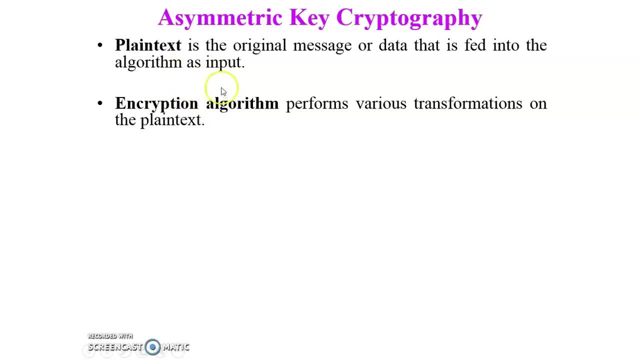 Either it is a public key or private key, So output of this algorithm is cipher text: Public and private keys. This is a pair of keys that have been selected so that, if one is used for encryption and the other is used for decryption, either public key is used for encryption. 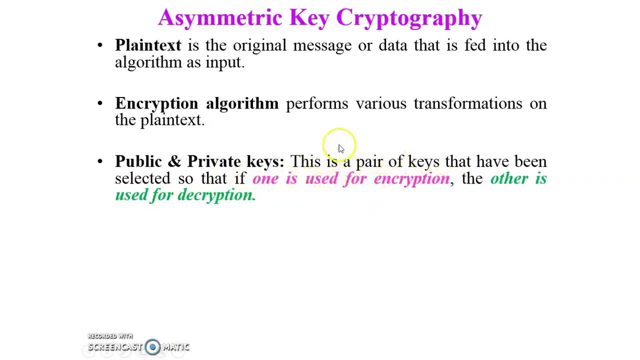 So So private key is used for decryption. either private key is used for encryption and then public key is used for decryption- Both the scenario we will discuss in this video- Cipher text. Cipher text is the unreadable message. It is the produced by encryption algorithm. We have already discussed about that. 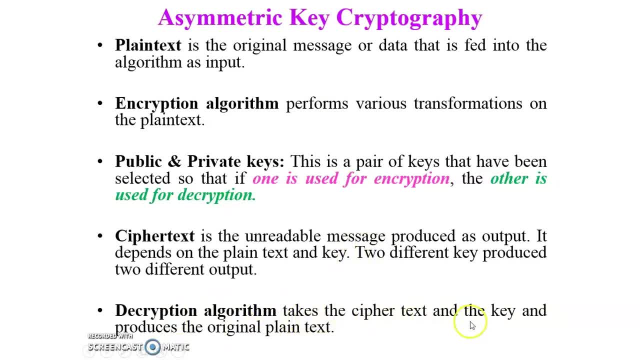 Decryption algorithm. It takes the cipher text and the key as an input and produce the original plain text. So encryption algorithm will be executed at the sender's side. So encryption algorithm will be executed at the sender's side. So encryption algorithm will be executed at the sender's side. 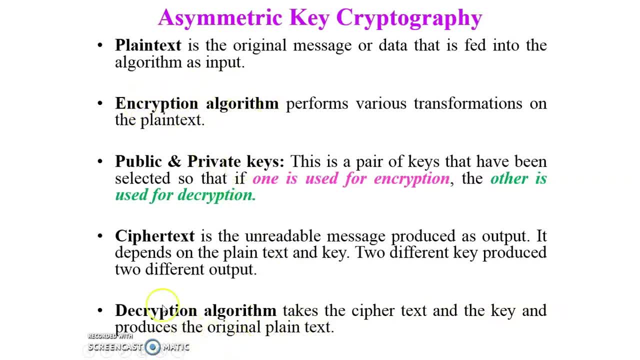 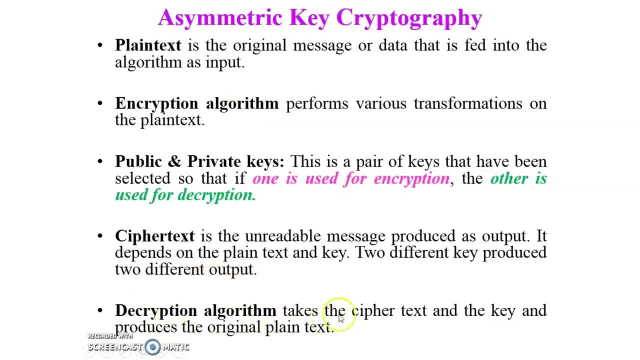 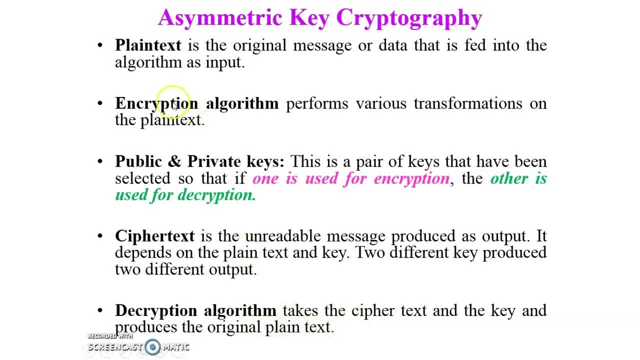 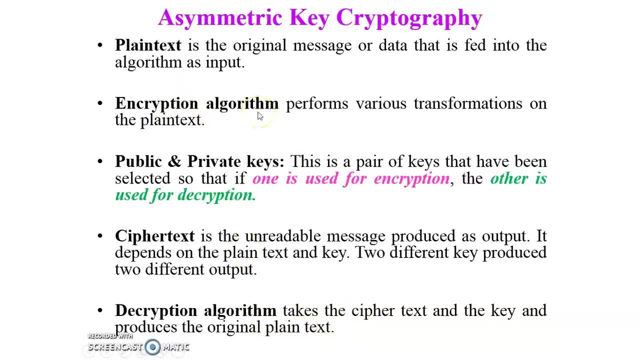 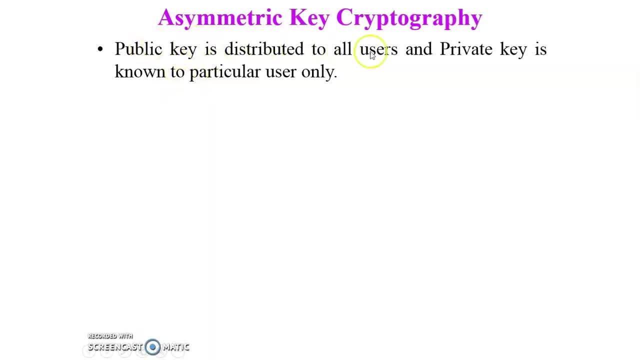 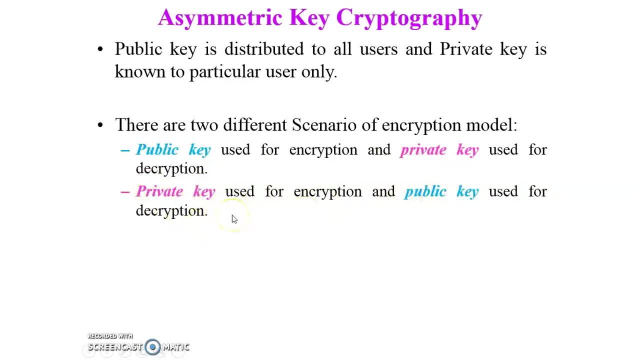 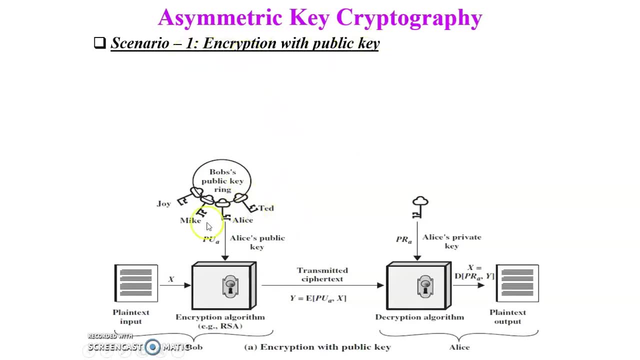 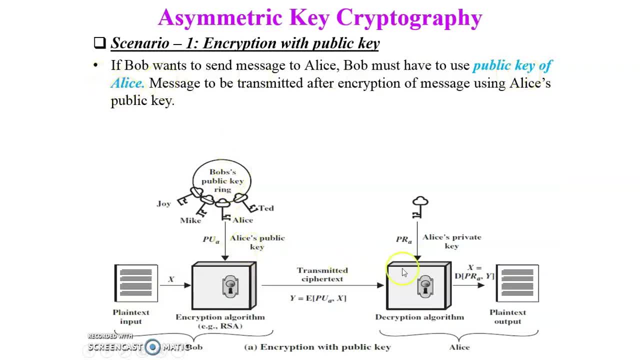 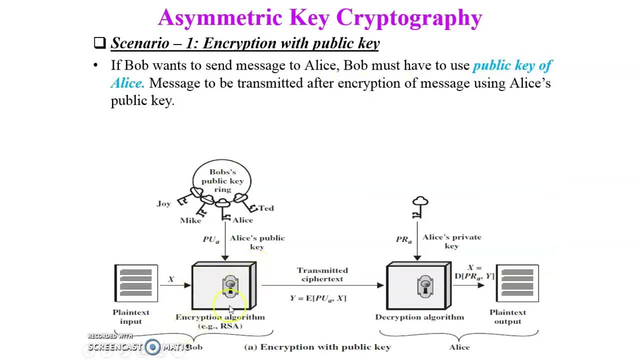 Alice public key after output of the encryption algorithm is Y and why it is called ciphertext. so ciphertext is transmitted to the receiver side. Alice has received message and she can decrypt the message using only her private key. now you can see over here: this is the PRA notation: PR is private key and a is 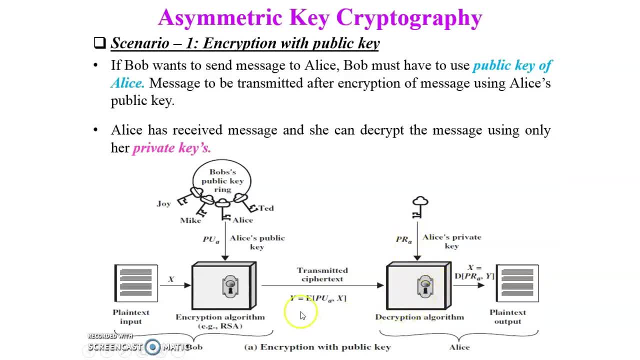 Alice private key. so decryption algorithm: input is ciphertext which is transmitted by Bob, and input is another. input is private key of Alice and it generate plaintext output. so this is the encryption with public key. mathematically, this scenario represented as public key of a, now PU of a, and the 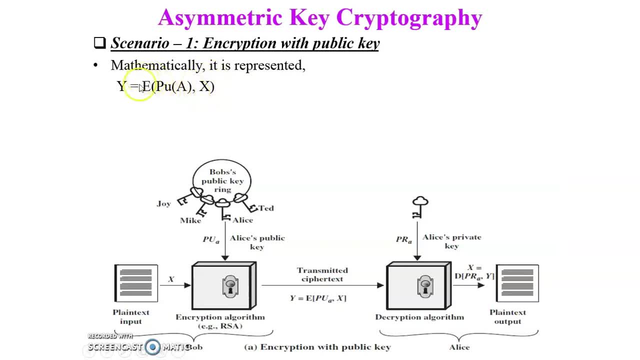 another input is original plaintext X and it is encrypted by encryption algorithm and it generates Y ciphertext and decryption process. D is the decryption of rhythm. in a decryption process, one input is Y, this is ciphertext transmitted by Bob, and another input is private key of Alice, so PR of a. so this is the decryption process and it. 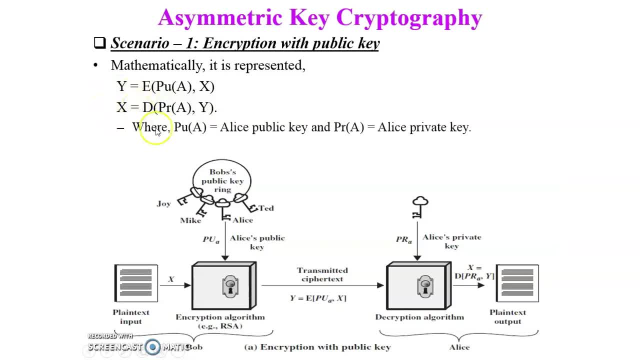 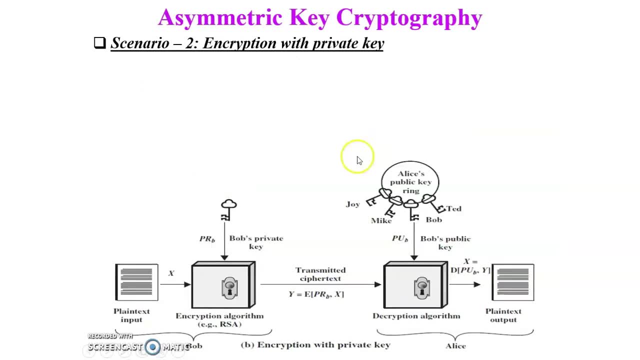 generates for regional plaintext X- now you can see over you- a is equal to Alice public key and PRA is equal to Alice private key. second scenario is another And second scenario: encryption with private key. In this figure you can see over here, this is Bob is the sender and Alice is the receiver Here. if Bob wants to send the message to Alice, now you can see over here- and Bob must have to use his own private key. 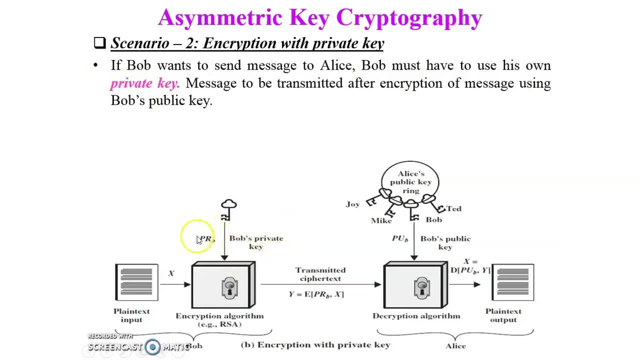 Now this is the Bob's private key. So we have right over here P R of B. So encryption algorithm, input is capital X and P R of B, private key of Bob Message to be transmitted after encryption of message using Bob's public key. So output of this encryption algorithm is capital Y and Y is transmitted to the receiver side through a secure channel. 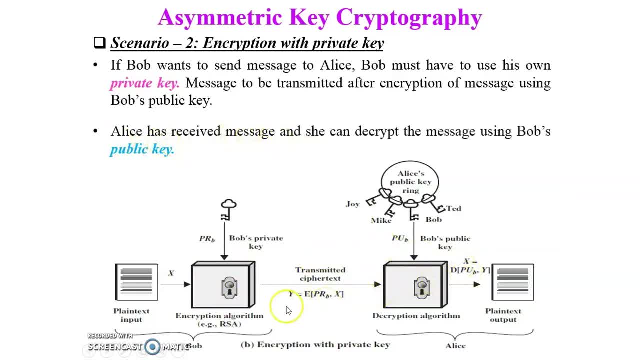 Next one: Alice has received the message. Now you can see over here. So Y is reached, So we can say at Alice side. So we can say at receiver side, So she can decrypt the message using Bob's public key, because Bob's public key is known by Alice. So here you can see over here. So decryption algorithm: P? U, B, comma, Y decryption algorithm used is used. So input of the decryption algorithm is public key of Bob, So it is P? U of B, and another input is Y ciphertext, So its output is original plaintext. 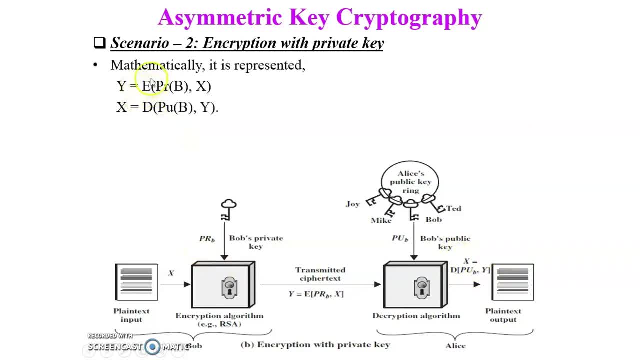 Now mathematically it is reproducible. Now you can see over here. This is the encryption process. It uses private key of Bob, So it is P? R of B, and another input is X. It generates ciphertext Y at decryption side, public key of B and ciphertext Y is the input of the decryption algorithm. It generates capital X. So it is the original plaintext message where P R B is equal to Bob's private key and P U B is equal to Bob's public key. 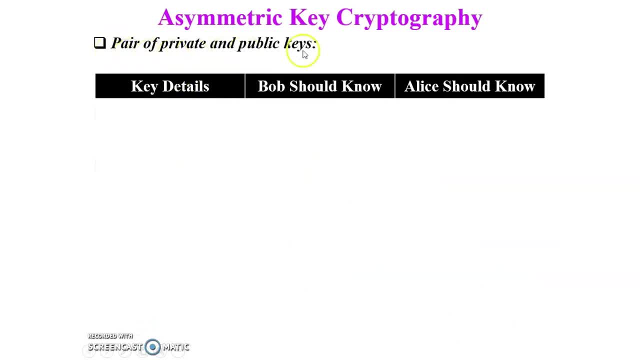 Now pair of private and public keys. So who will know whose private key and whose public key? Now this is the key detail. See one by one, Bob's private key. So it is denoted by P R of B. So Bob must know, but Alice does not know about Bob's private key. 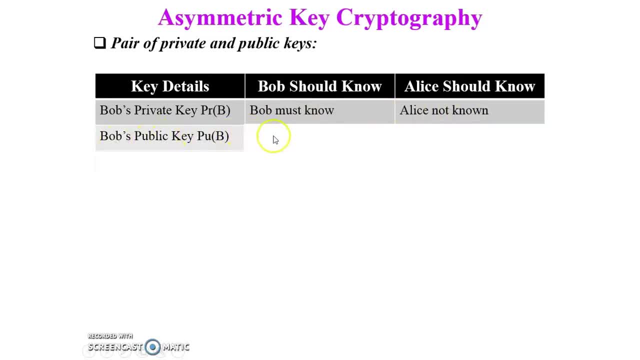 Next one, Bob, public key. So it is P? U of B, So public key is known by Alice also. So this is Bob must know, also known by alice. so this is public key. so bob and alice both are known, same as alice, private key. so bob not known and alice must know. so this is private key which is not shared. 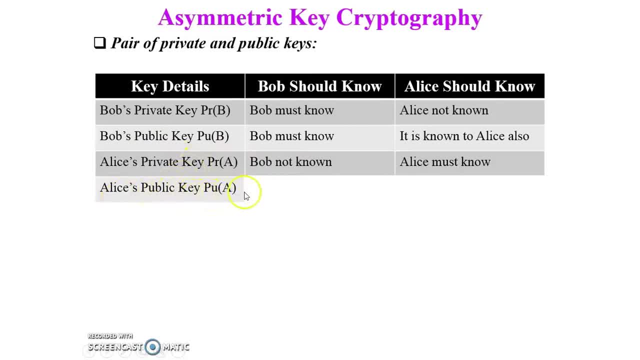 with bob alice public key pu of a. so this is public key. so both user known the public key, it is known to bob and alice must know. uh, for example, uh, sorry, a famous example of asymmetric key cryptography is rsa algorithm, the reverse samir and aderman and defy hellman. 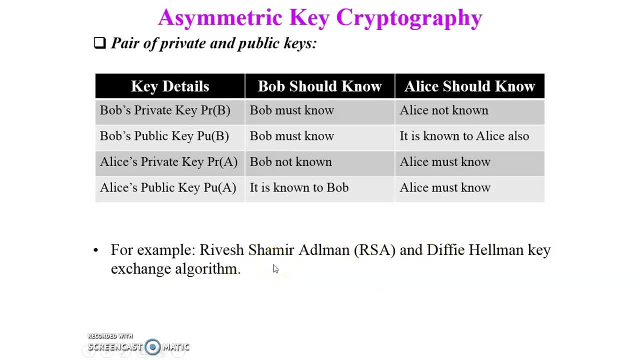 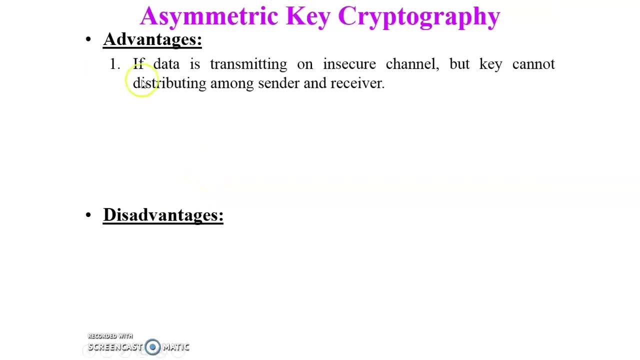 key exchange algorithm. these are the famous algorithm of the asymmetric key cryptography. now, advantage and disadvantage of asymmetric key cryptography. first one: if data is transmitting on insecure channel but key cannot distribute among the sender and receiver. if a hacker or attacker will get the message or capture the message from the insecure channel, but they cannot decrypt the message, separate key. 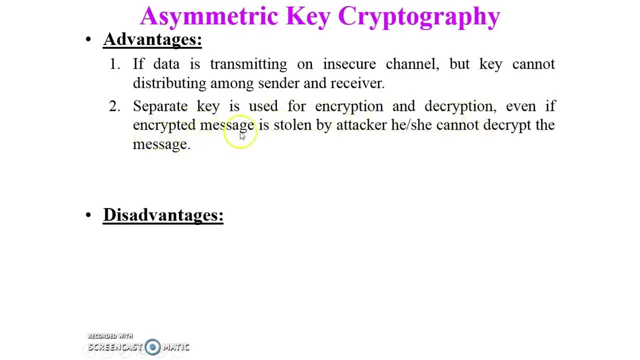 is used for encryption and decryption, even if encrypted message is stolen by attacker or he or she cannot decrypt the message easily. easy to user. for user disadvantage: asymmetric key use more resource in compared to symmetric key cryptography. more mathematical calculation required. so this is the biggest disadvantage of the asymmetric key cryptography: slower in compared to symmetric key cryptography. 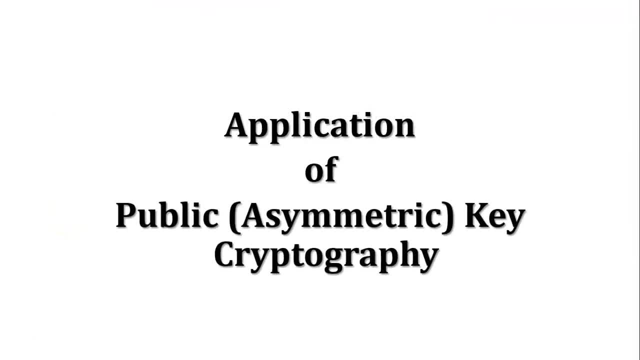 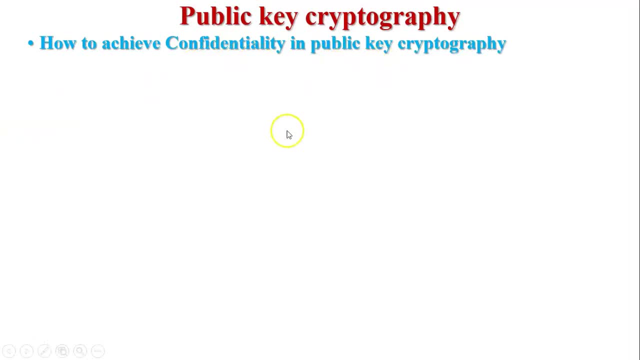 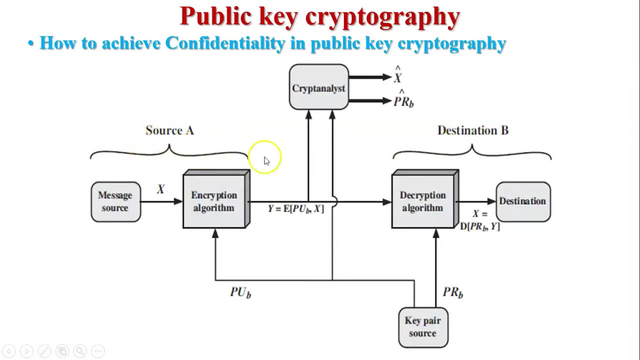 now discuss about application of public or asymmetric key cryptography. now how to achieve confidentiality in public key cryptography? now see this figure: this is sender and this is receiver. so we can say it is source a and this is the receiver. so we can say it is source a and this is destination b message source. so this is x is the original original message. 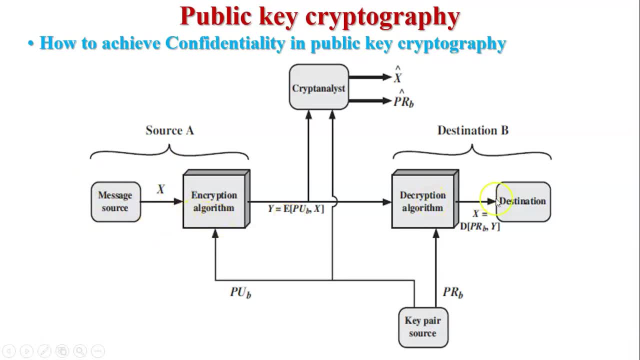 and original message will be send by the sender to the receiver. so before sending this message, encryption algorithm is used and it generates cipher text. now what is the input of encryption algorithm? that is original plain text message and pub-. p-u-b is public key of b. now here: 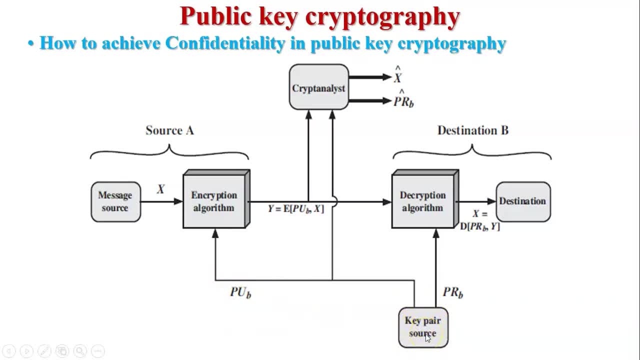 you can see in the figure, this is the first index of decryption and the last index of figure. this is key pair source. it means there are two key will be generated at the destination or we can say receiver side. one is public key of the receiver or destination, public key will be said. 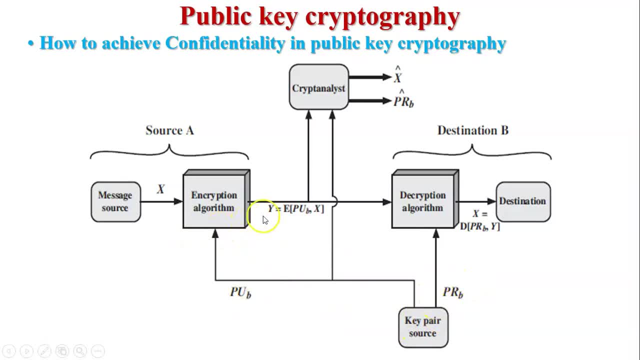 with the sender and private key remain secret. now here y is equal to encryption of pubx. it means x will be encrypted using the public key of b and it generates ciphertext. now ciphertext will be sent to the receiver side. now we can say: this ciphertext will be decrypted by only one and 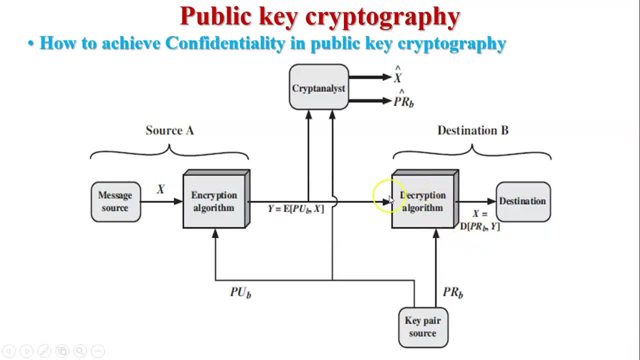 only key, private key of b. now here decryption algorithm is used. input of the decryption algorithm is ciphertext y and private key b. it generates original plaintext x and read by the destination. it means any of the user in the network which is connected to the source and destination will be sent to the receiver side. now we can say this ciphertext will be decrypted. 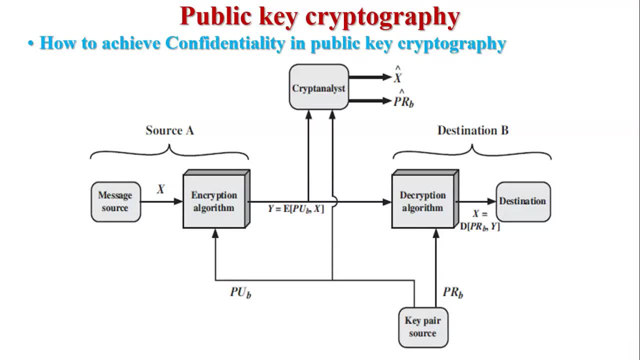 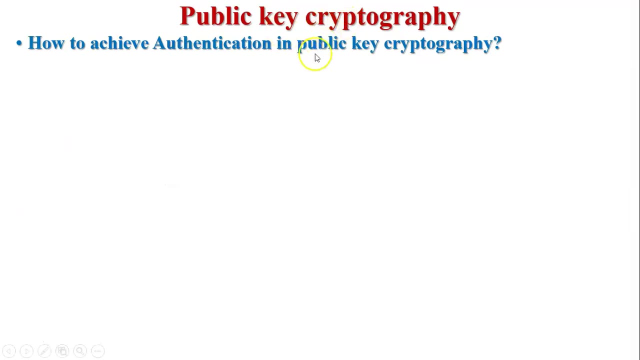 by only one and only key, private key of b and destination b will not decrypt this message. so, as per the definition of confidentiality, we can say a message should be known by only sender and receiver. it means achieve confidential. next, how to achieve authentication in public key cryptography. 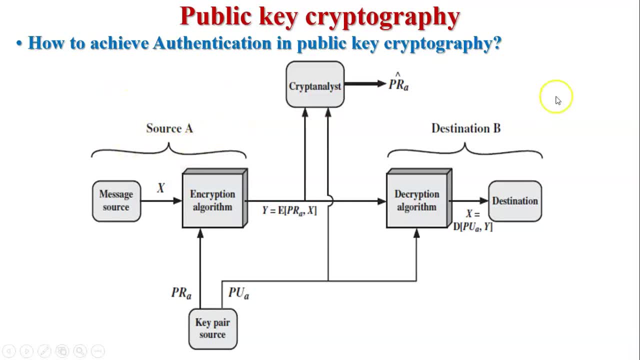 now see this figure. this is the source a- we can say it is sender, and destination b, it is receiver source. or we can say sender- sender wants to send data to the receiver. now, message source this is x is the original plaintext. so input of the encryption algorithm is original message and original message will be encrypted by private key of. 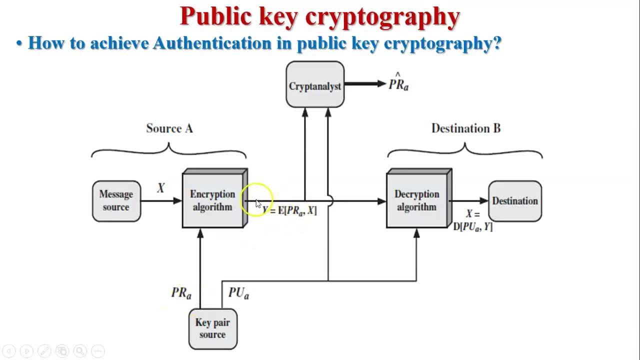 sender, because this is pra. now it generates ciphertext y. now you can see this equation. now y will be put on the secure communication channel, so this message will be received by all the network user. So we can say: decryption algorithm is used at the receiver side and during the decryption algorithm input is Y, ciphertext Y and public key of A. So all the users on the network who have public key of A, that all the users decrypt that data Here. destination decrypt the data using the public key of A. 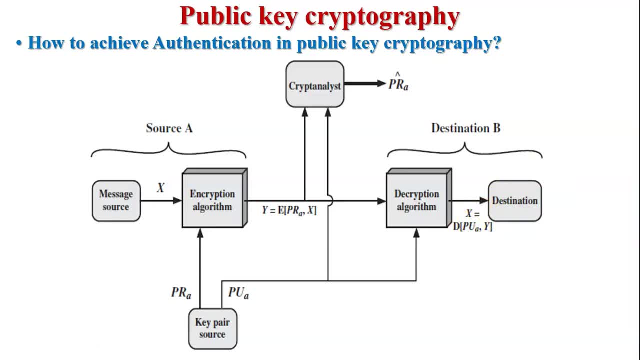 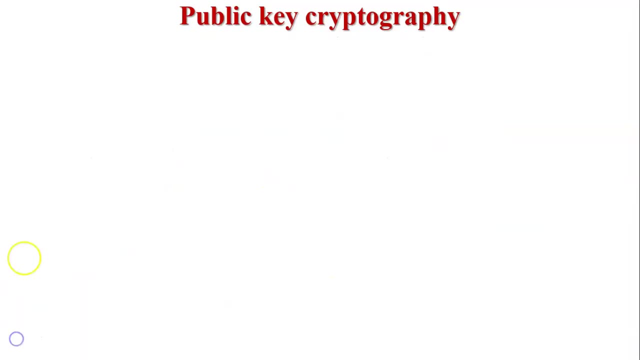 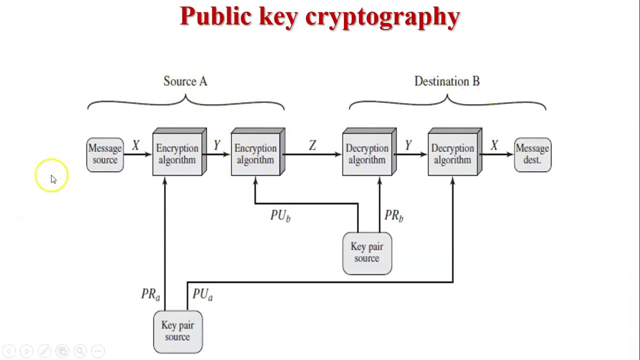 So as per the definition of authentication, we can say: receiver can receive the data and check whether data was sent by original sender or not. So using this figure, we can achieve authentication in public key cryptography. Now check next diagram Here in next diagram, this is sender and this is receiver. Sender sends original message. So before sending this message, it is encrypted. 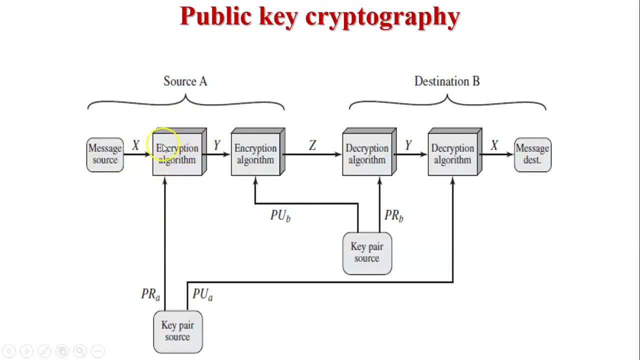 By encryption algorithm. So here there are two encryption algorithm is used. using first encryption algorithm, The input of the encryption algorithm is original message X and private key A. We can say it is private key of the sender, So it generates ciphertext Y. In second encryption algorithm, input is first generated, ciphertext Y, and it will be encrypted using the public key of B. 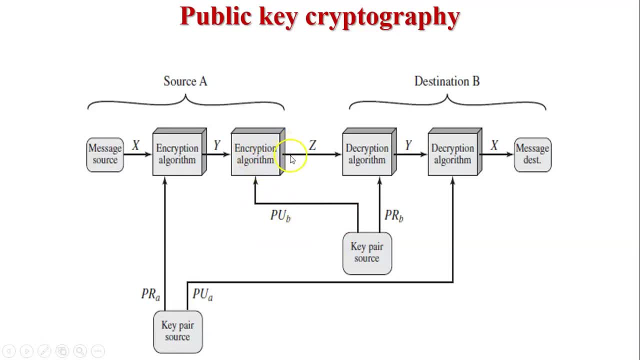 We can say it is private key of B. It is the receiver's public key. It generates final ciphertext: Z. Z will be sent to the receiver and receiver first use the decryption algorithm. It will be decrypted by private key of B because last encryption is done by public key of B. 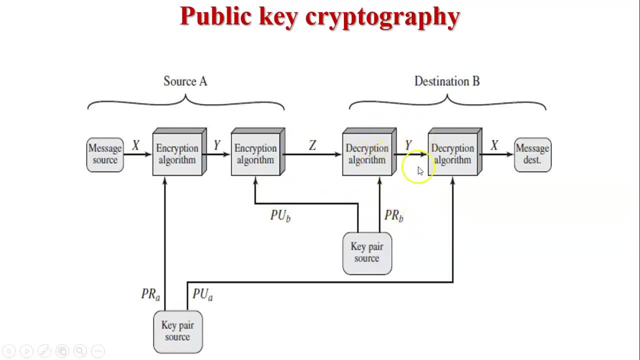 So private key of B decrypted and it generates Y. Y will be again decrypted using the public key of A. It generates original message X. So here we can say: We will achieve confidentiality and using this key pair we will achieve authentication. So we can say: here confidentiality and authentication are achieved in this figure. 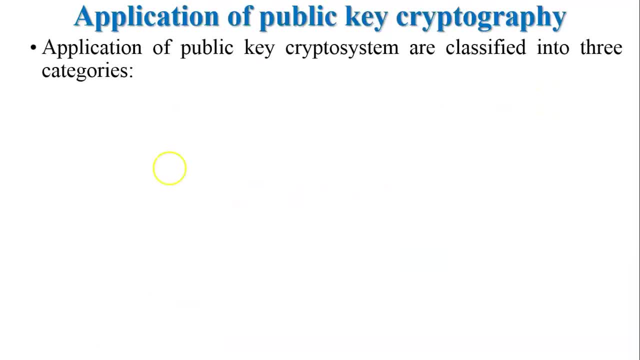 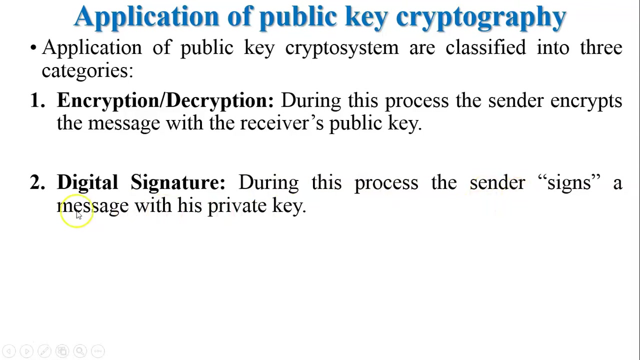 Next, application of public key cryptography. Application of public key crypto system are classified into three categories. First one is encryption decryption, So this application will be also apply at symmetric key cryptography- Encryption- decryption. during this process, the sender encrypt the message with the receiver's public key. second one: digital signature. during this process, the sender signs the message with his private key. 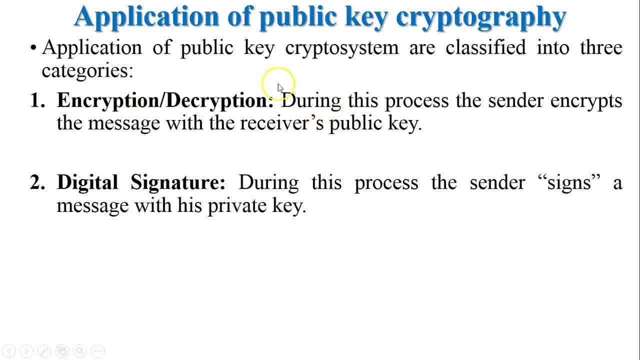 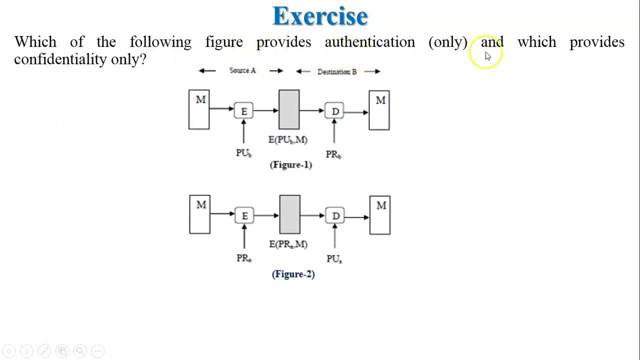 So we can say: this is using encryption decryption. we can achieve confidentiality. using digital signature we can achieve authentication. key exchange: both sender and receiver cooperate to exchange a session key, typically for conventional encryption. Now exercise which of the following figure provides authentication only and which provides confidentiality only. 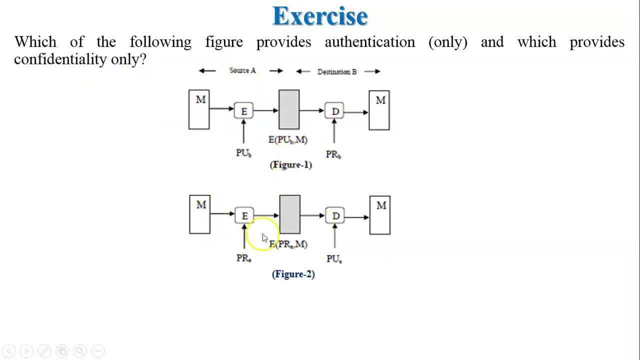 Now, this is figure one and this is figure two, Where M is the plaintext in both the figures. E is the encryption function, D is the decryption function. PRA and PRB are private keys of source a and destination b Respectively. 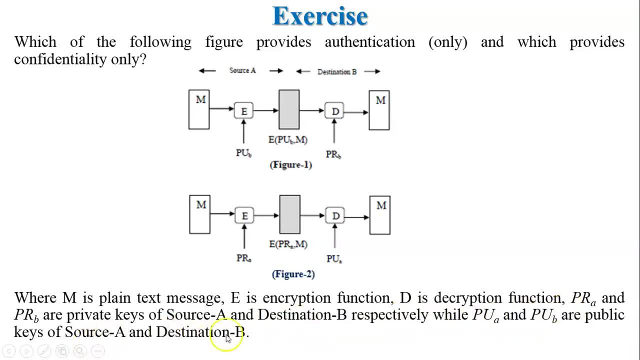 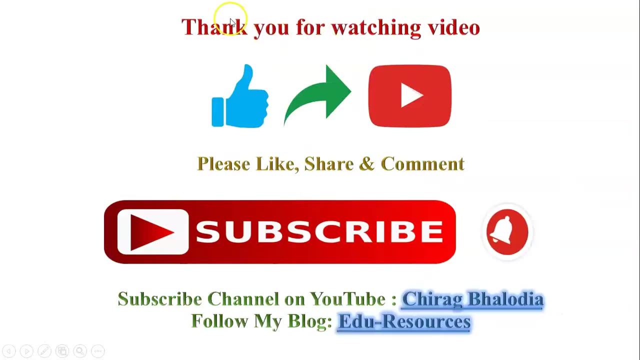 While PUA and PUBG are the public keys of source A, of source A and destination B. So you have to find which figure provides confidentiality and which figure provides authentication. So write your answer in comment section. Thank you for watching this video. please like share. 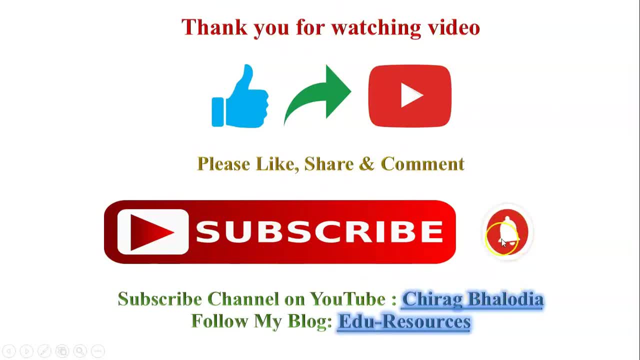 and comment. Subscribe my channel on YouTube, Chirag Balodia. Press bell icon to get new video notification. Follow my blog: EDU resources. Thank you.